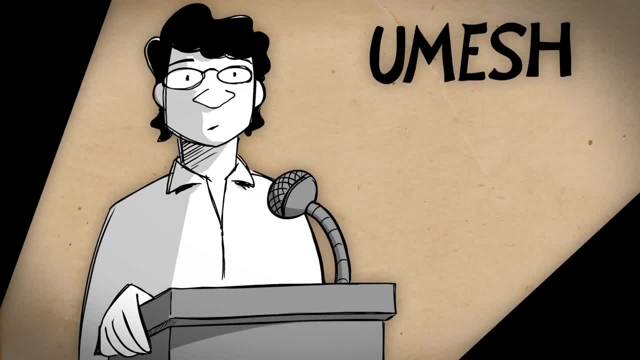 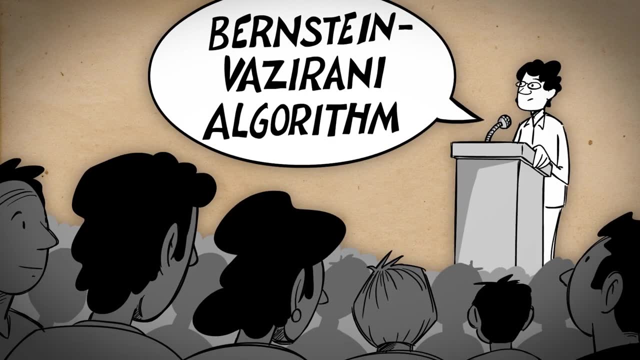 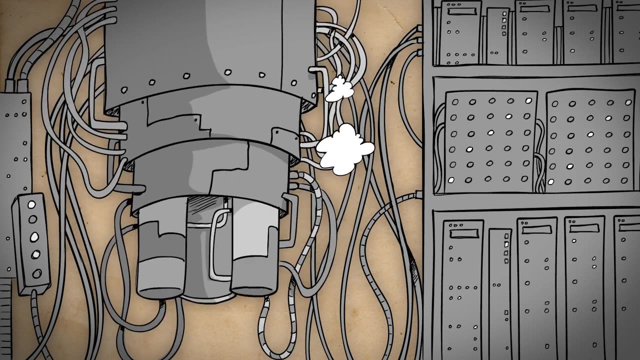 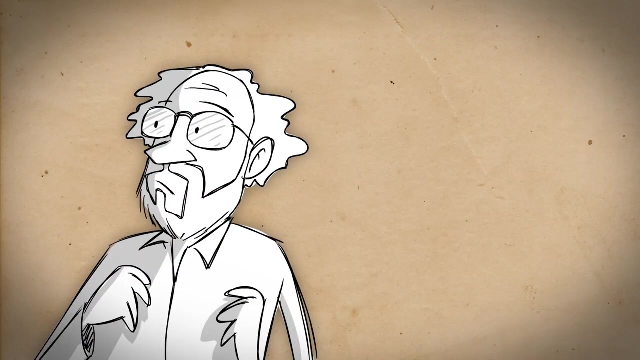 In 1992, Umesh Vazirani came to Bell Labs and he gave his talk on Bernstein and Vazirani, where he put quantum Turing machines into a mathematically rigorous framework which seemed to run faster on a quantum Turing machine than on a classical computer. So that really intrigued me and I 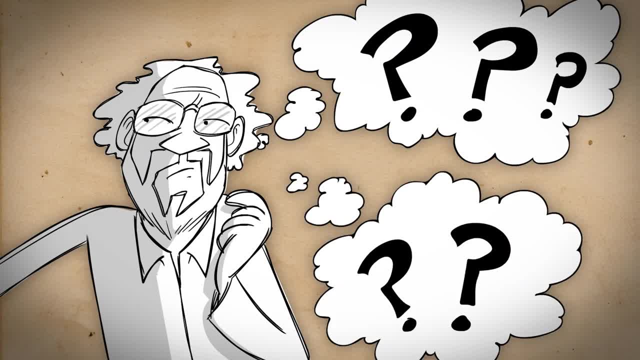 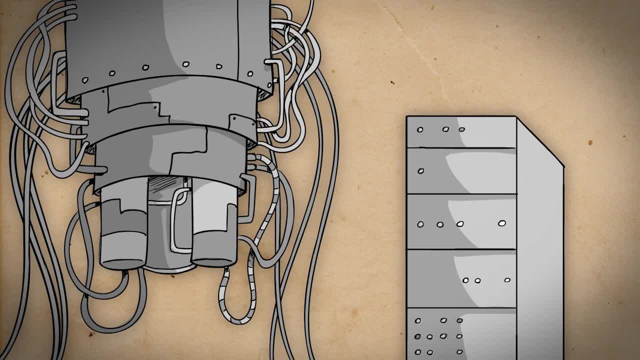 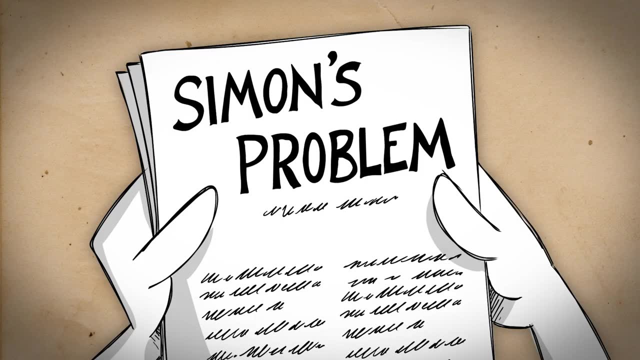 started thinking about whether there were any more convincing problems that could be done on a quantum computer much more efficiently than on a classical computer. I didn't get anywhere on this question until I saw a paper of Dan Simons, So Simons' problem was given a function. 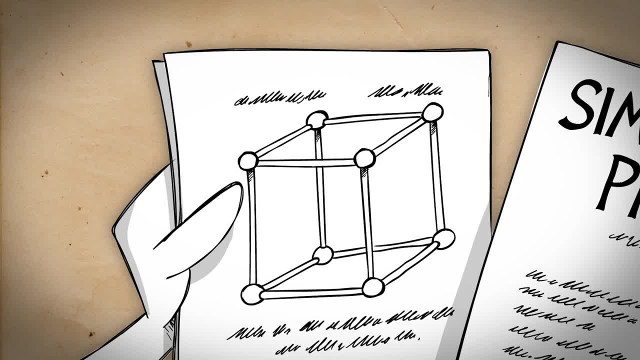 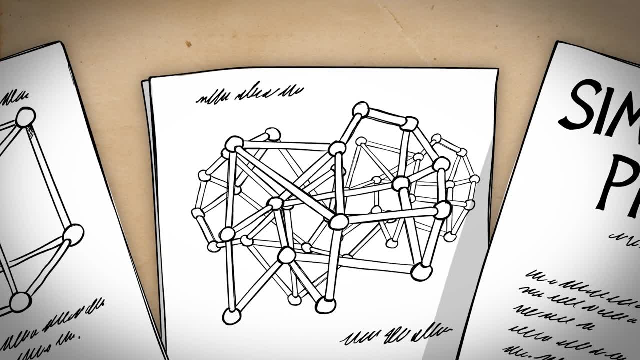 like this, which you only can access as an oracle, find a period. So here's a three-dimensional cube, in which case the problem is trivial. but if you have a five hundred dimensional cube, it suddenly gets very hard. So a similar thing holds for factoring. If you can factor, 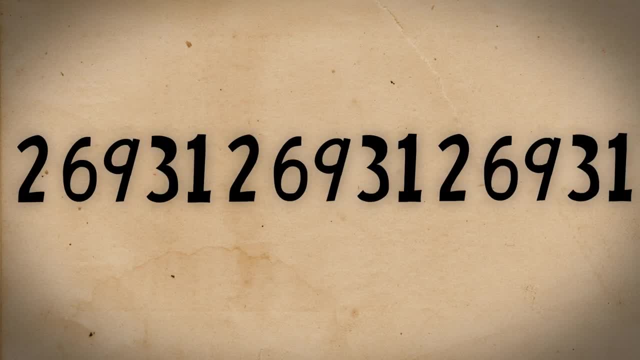 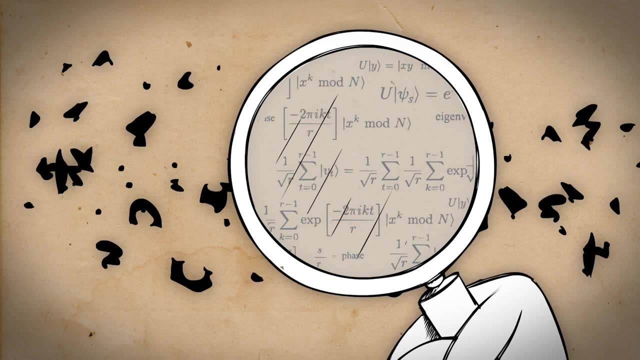 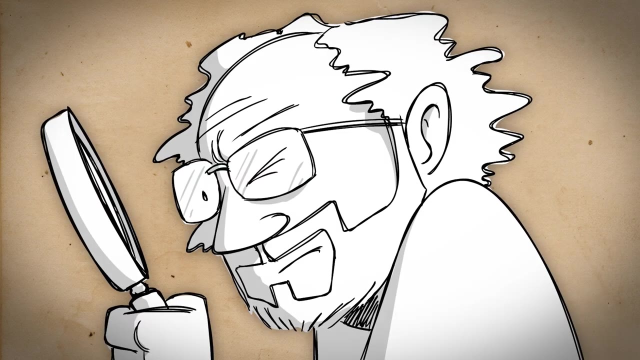 large numbers rapidly, you can break the RSA crypto system. I knew that the Fourier transform was very important for finding periods, so I figured out how to take the Fourier transform on a quantum computer over exponentially large period, and then I figured out how to apply it to Sol-get discrete. 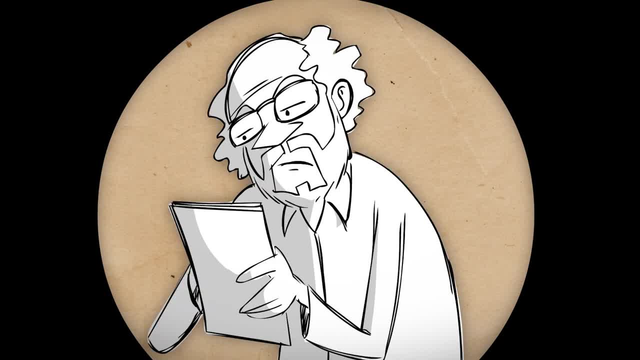 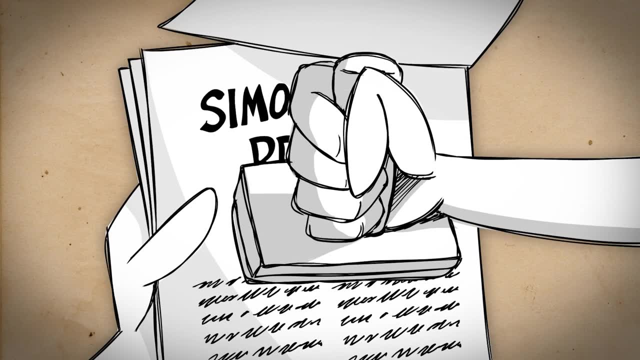 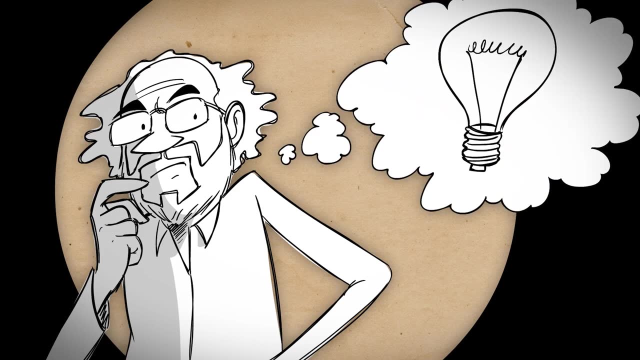 log. And there's a very embarrassing thing here, which is that I had seen Simon's paper when I was on the program committee. We rejected Simon's paper from the conference and then, before it actually appeared, I realized I could use the idea. So I called Simon and, you know, got him to send my paper. 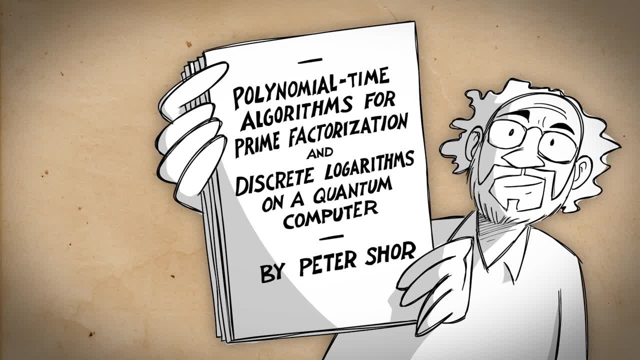 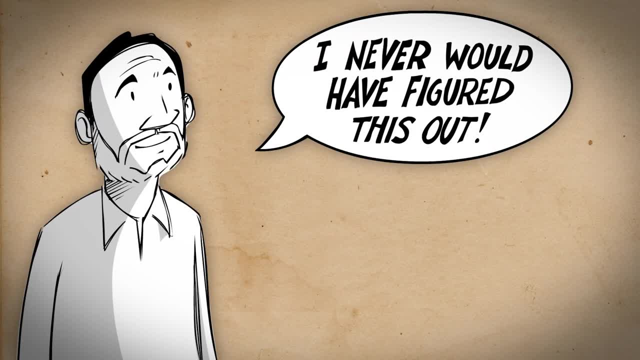 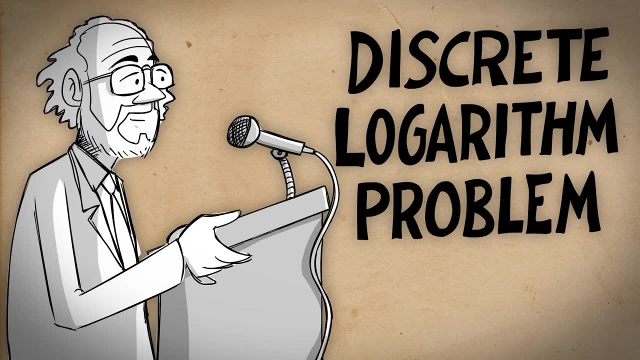 and um so I would have a legitimate copy. and then I went and um wrote my paper and Simon said that he never would have figured this out, so he didn't really mind that that. Once I'd solved the discrete log problem, I gave a talk about it at Bell Labs, which has a very active audience. The 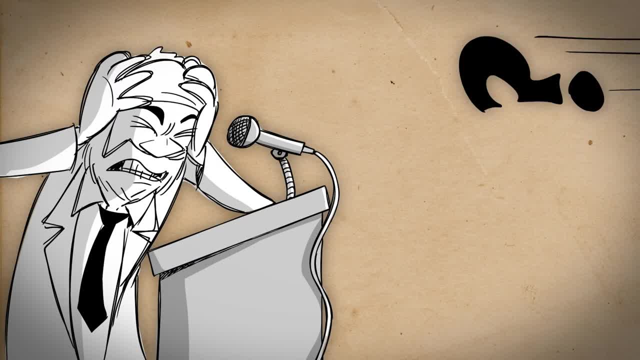 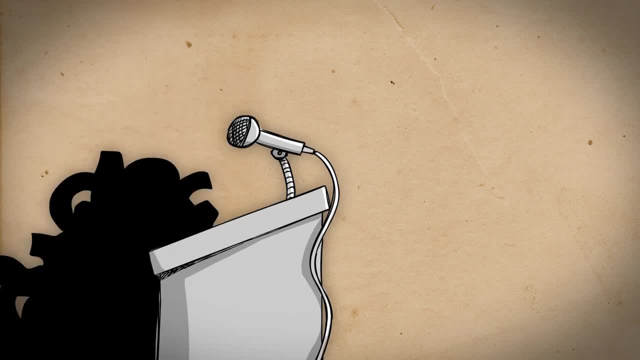 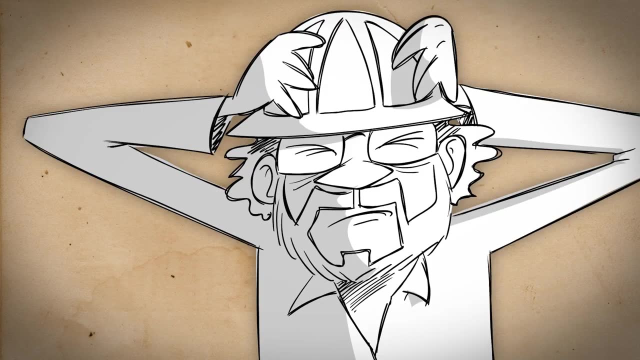 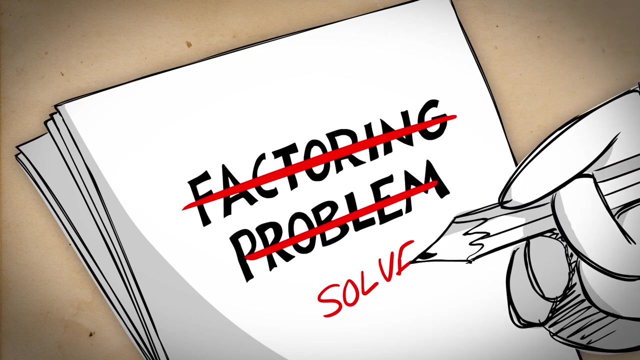 speaker gets constantly pelted by questions and there have been at least one or two occasions when people have never been able to get through more than the first two or three of their transparencies. Actually, it went very well. I went back to work and I managed to solve the factoring problem a few days later, So five days. 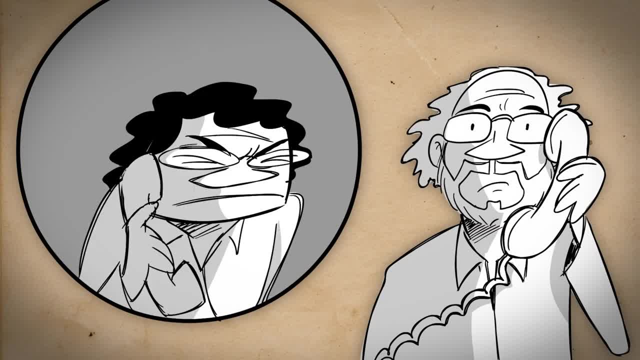 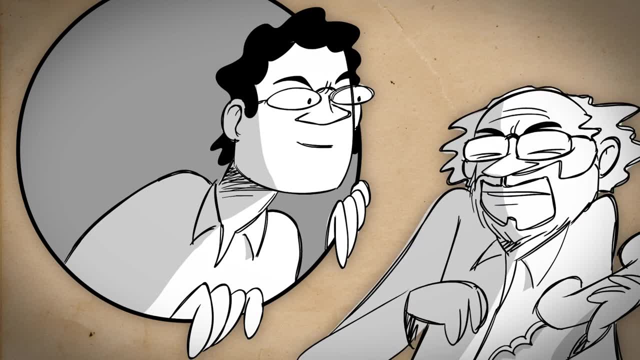 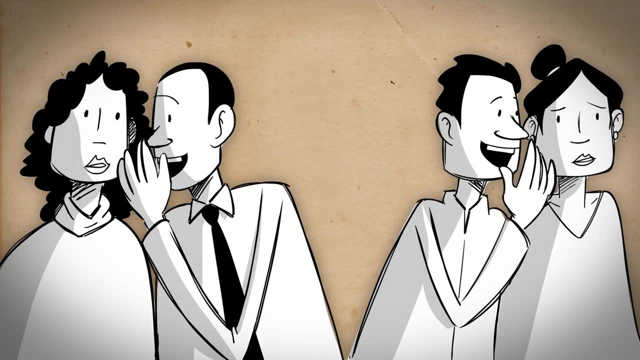 after my call I got a call from Umesh Vazirani saying I hear you can factor on a quantum computer. tell me how it works. I told him that I how to factor large numbers on a quantum computer. The rumor mill must have spread the result very rapidly. And second, if you know the old children's 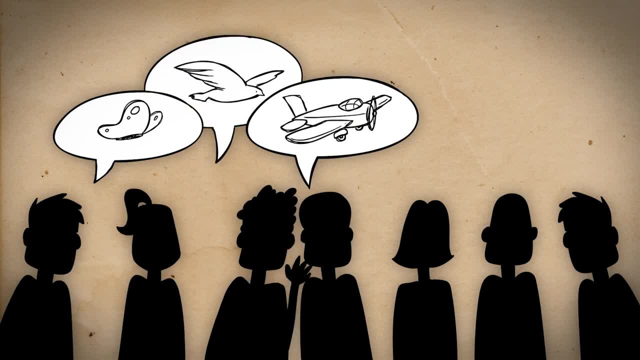 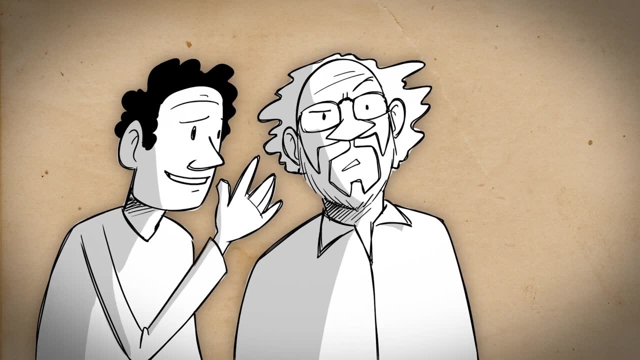 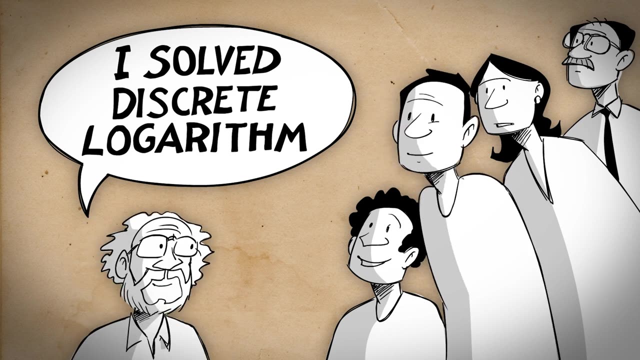 game of telephone. one person whispers something to the next, whispers something to the next whispers something to the next, and it's completely changed by the time it gets around to the first person. Well, I had told everyone I'd solved discrete log and I don't think I told anyone other than maybe. 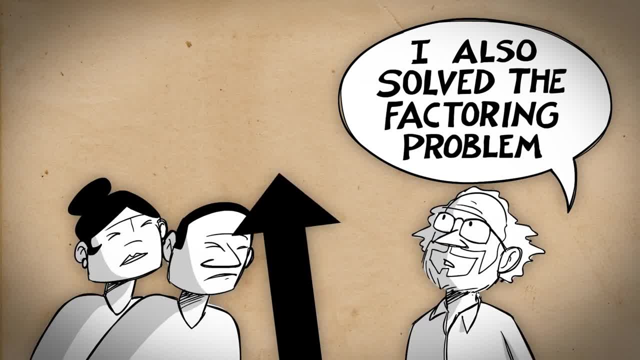 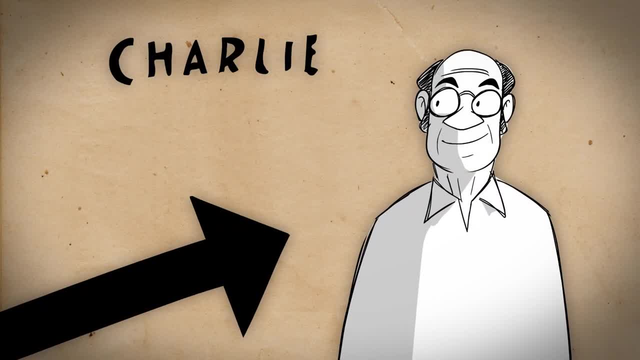 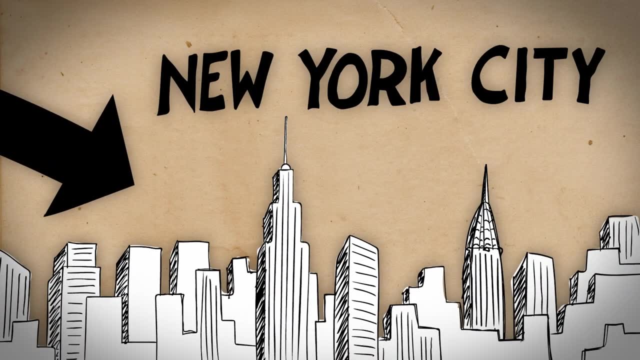 one or two people that I'd been able to solve factoring as well, but somehow the rumor changed. discrete log to factoring. The first time I talked about that with anybody was Charlie Bennett. There was a Columbia 30 Day, which was held twice a year in New York City and there was one in late April, and Charlie Bennett. 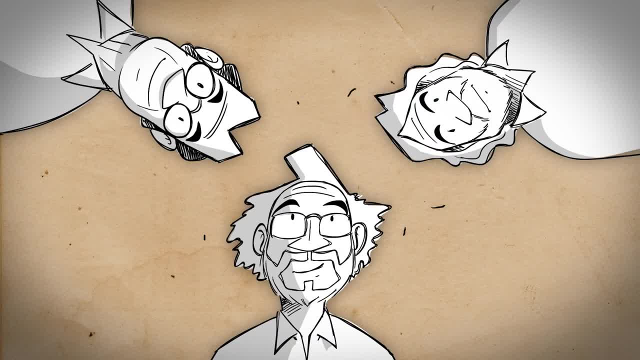 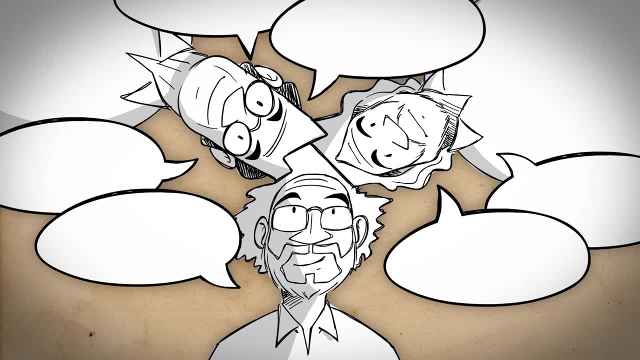 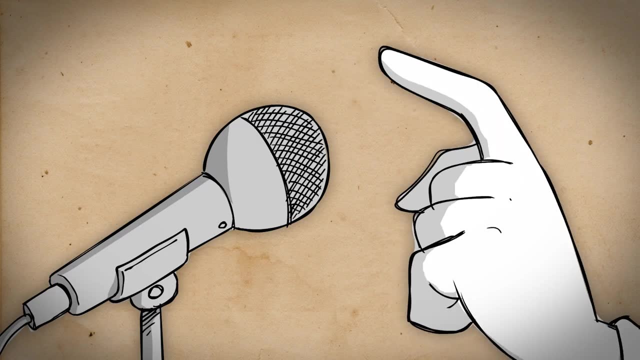 and John Smolin and I arranged to get together at the 30 day and I could talk about the factoring algorithm to him and then he explained some interesting things about quantum puzzles and quantum information to me. Then next thing was I gave a conference at the Cornell algorithmic number theory symposium, which I think was the 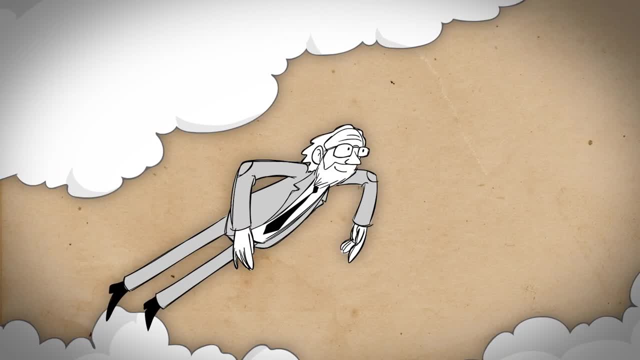 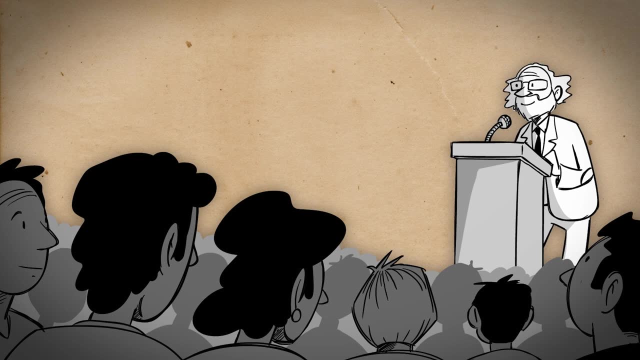 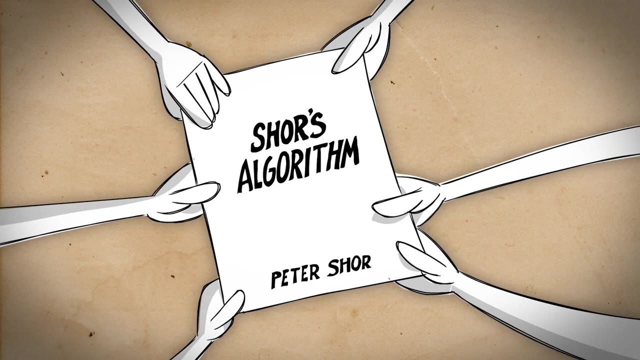 first of a annual conference and so I flew up and gave my talk and, um, there was someone from the NSA there who came up and asked me questions about it afterwards. You know I was deluged for by requests for my paper. I got interviewed by a bunch of magazines. 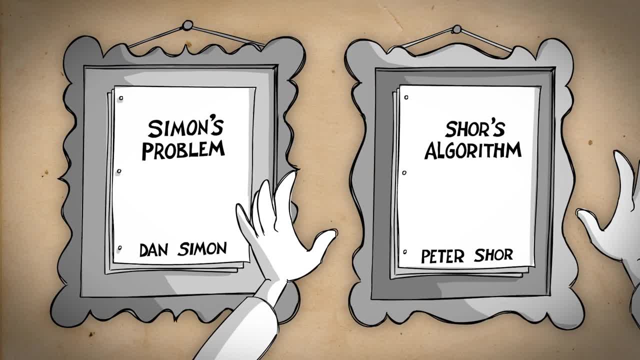 and both Simon's paper and my paper got accepted to Fox and I presented the result there.